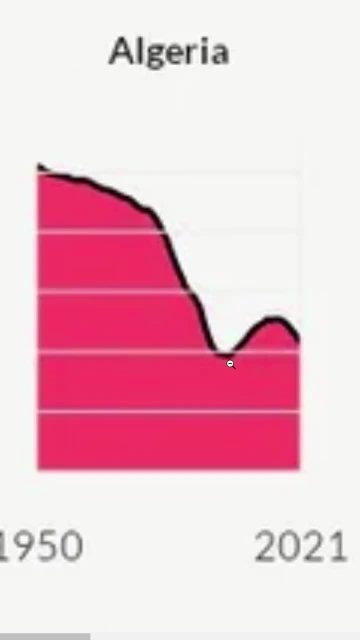 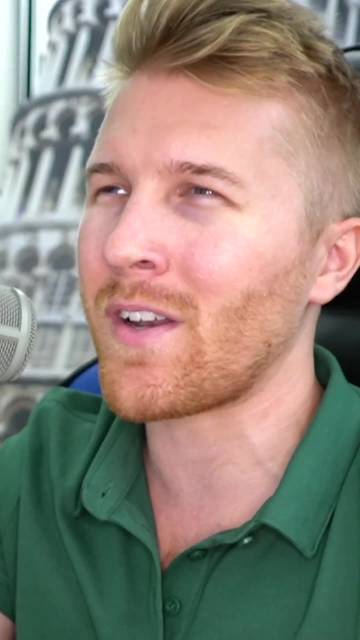 Afghanistan remained pretty high up until recently. Interesting that Algeria had like kind of a comeback, but then it dipped back down. I remember seeing all these graphs when I was a kid that, like overpopulation, was going to be an insane problem one day. 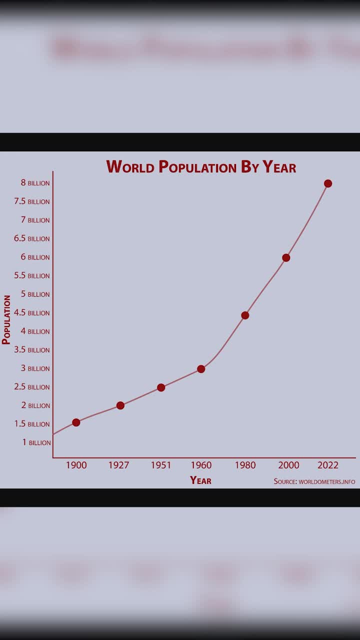 Not that it won't, but they just assumed that birth rates were going to remain the same from like the 1950s. Like we're about to have 50 billion people living on Earth in 2030.. 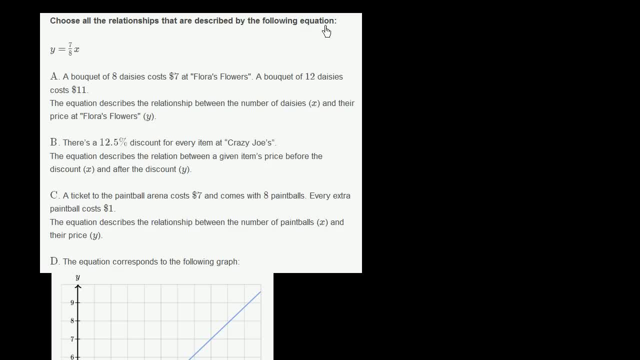 Choose all the relationships that are described by the following equation: y is equal to 7 eighths x. All right, let's look at these relationships. Relationship A: a bouquet of eight daisies costs $7 at Flora's Flowers. 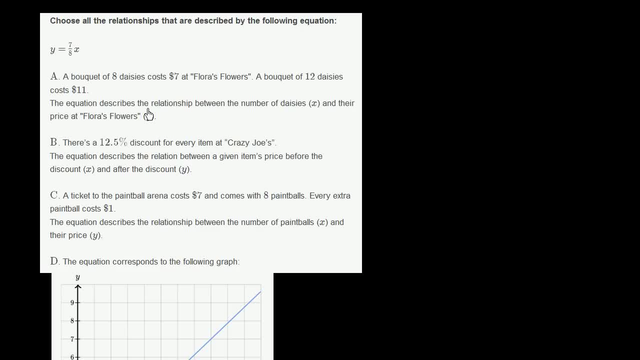 A bouquet of 12 daisies costs $11.. The equation describes the relationship between the number of daisies, x, and their price at Flora's Flowers y. So let's look at scenario A. So our x is the number of daisies and our y is their price. 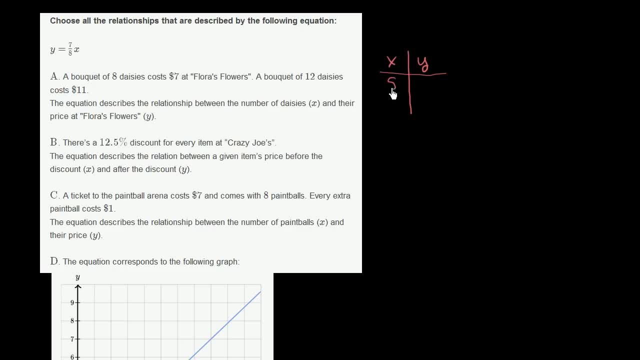 Our y is the price. So when we get eight daisies, they say it costs us $7.. When we get 12 daisies, they tell us that it costs $11.. So let's see whether this relationship right over here. 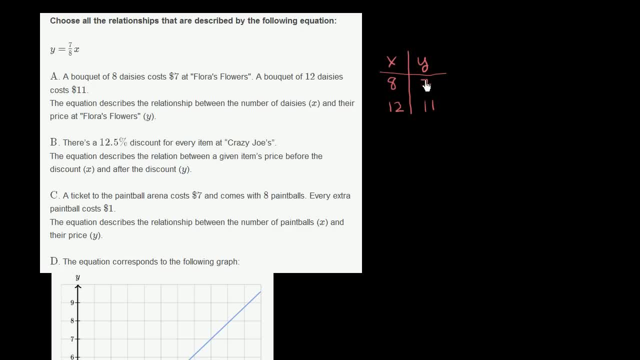 is the same as this relationship right over here. So if I were to take, so let me write this right over here. So here it says y needs to be equal to 7 eighths x. So let's figure out what 7 eighths x is equal to.